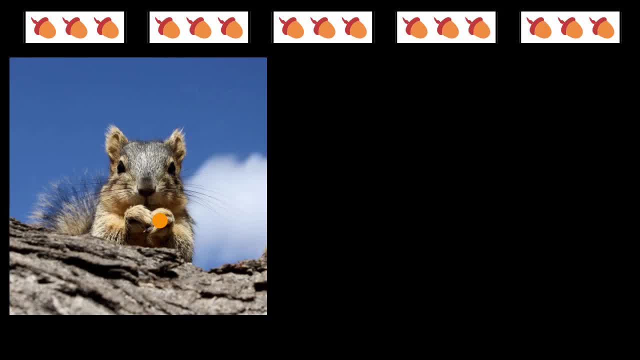 Our squirrel friend here likes to collect acorns because really that's how he is able to live, And, let's say, every day he collects exactly three acorns, And so what I'm curious about is how many acorns will he have after doing this for five days? 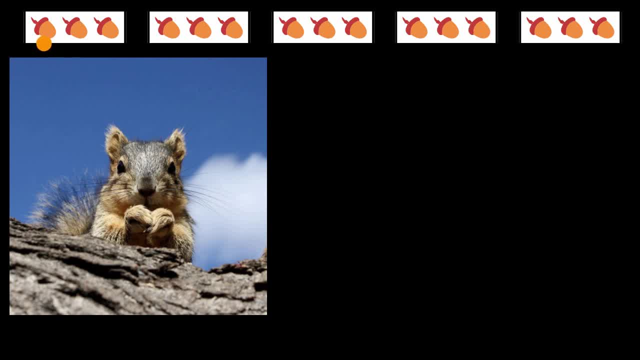 So one way to think about it is: every day he is able to collect a group of three acorns. So you could view this as maybe what he's able to collect in day one, And then in day two he's able to collect a second group of three acorns. 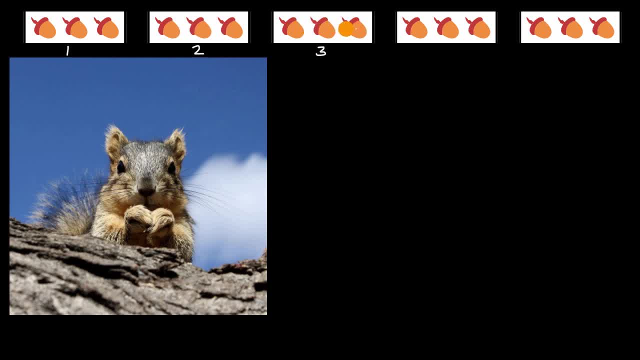 In day three he's able to collect another group of three acorns, And every day it's an equal number of acorns that he's collecting. On the fourth day, another three. On the fifth day, another three, And so, if you were curious, how many total acorns? 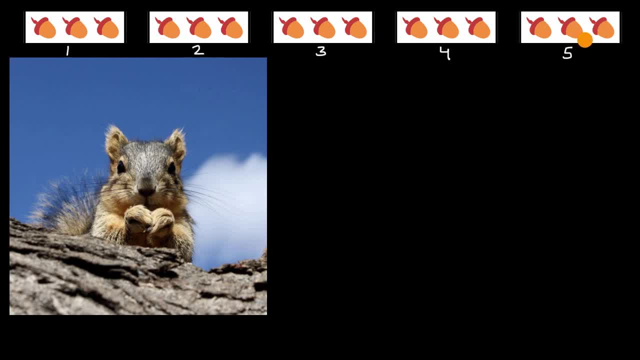 he's collected. well, you could just count them up. Or you could think about: well, he's got five groups of three acorns, five equal groups of three acorns, So you could say: five groups of three acorns, three acorns. 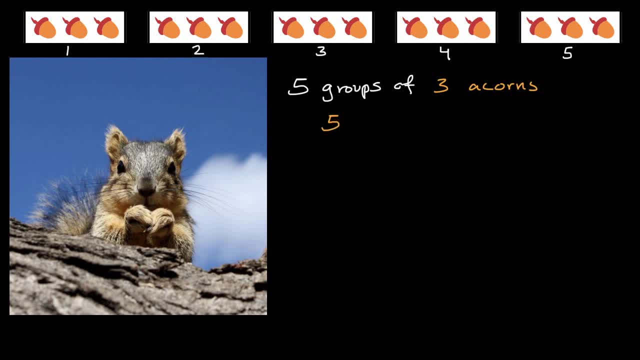 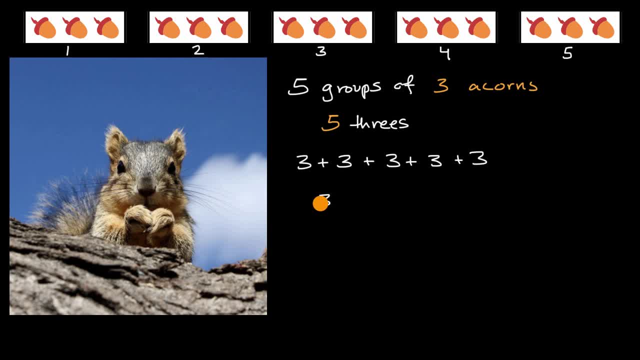 you could skip count by three. So this would be three, six, nine, 12,, 15.. Because we add three, we get to six. We add another three, we get to nine. We add another three, we get to 12.. 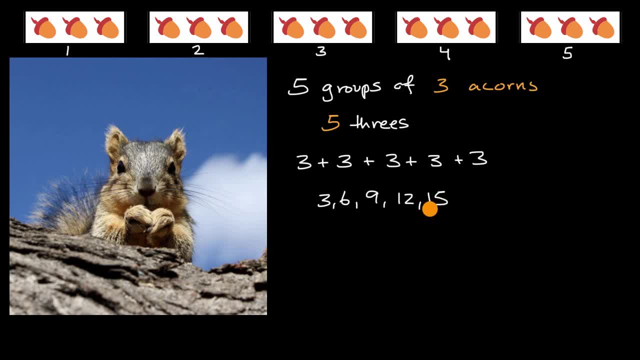 We add another three, we get to 15.. And so this would be a way of recognizing that you have 15 acorns. But we're starting to touch on one of the most fundamental ideas in all of mathematics. In fact, we actually are applying it. 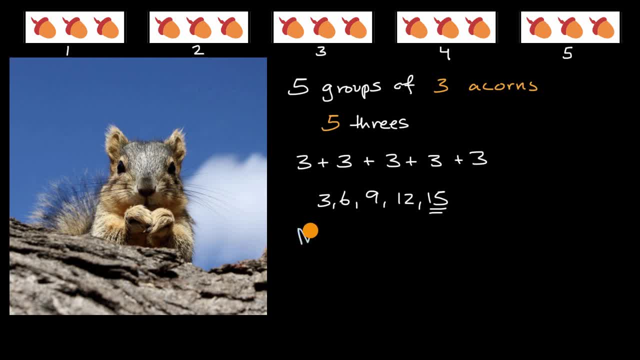 we just haven't used the word, And that's: we are multiplying, We are using, We are using multiplication. All multiplication is is this notion of multiple, equal groups of something. So here, one way to express what we just did, is we just when we said five, threes.